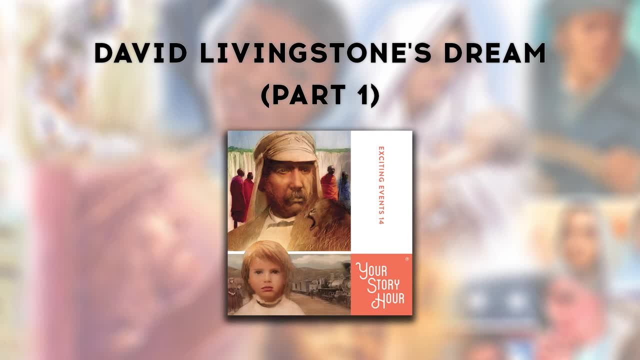 That's right. He eventually spent more than 30 years exploring Africa, paving the path for other missionaries to follow in his footsteps, And in the process he learned many of the native languages. like Setswana, Africa was a vibrant and thriving continent, full of languages and cultures and cities. 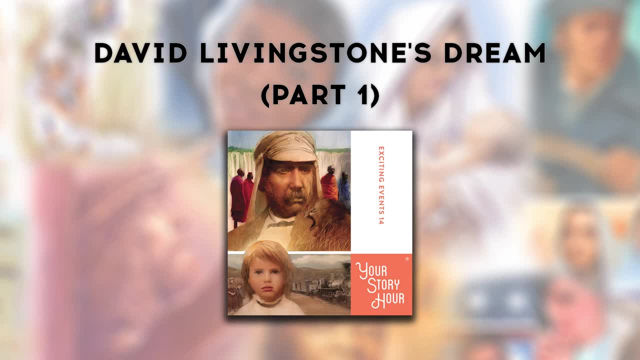 Africa was a vibrant and thriving continent, full of languages and cities, But back in the 1800s, people from Europe believed that cultures different from their own were uncivilized. You might hear that word in the story a couple of times. boys and girls, since we try to make our stories accurate to history. 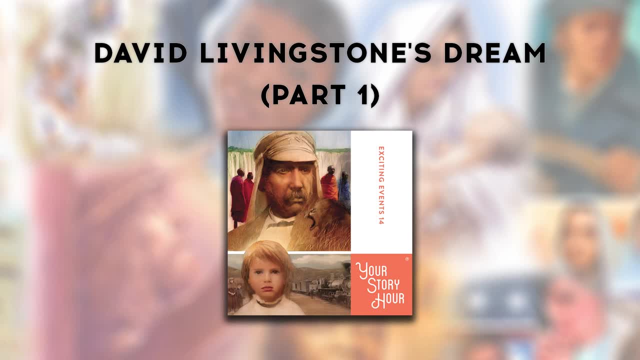 Mm-hmm. However, we want you to know that just because something's different doesn't make it bad or inferior. Differences are wonderful, Absolutely. Choirs create harmony by people singing the different parts, and the prettiest bouquets are those that have lots of different kinds of flowers. 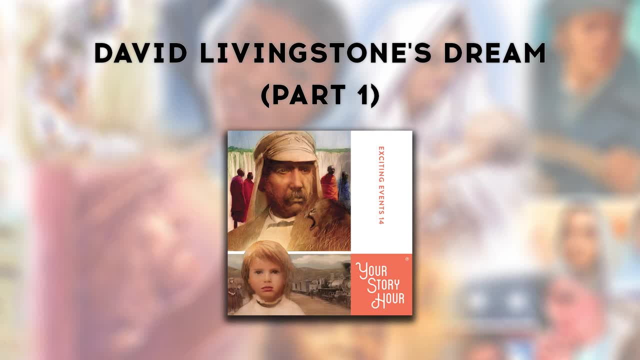 And speaking of things that are different, many of the languages that would have been spoken in this story are different and we wouldn't understand them. So, to make things easier, everyone will speak in English. Sounds good to me. Aunt Nikki, Now I think you know everything you need to know before we get started. 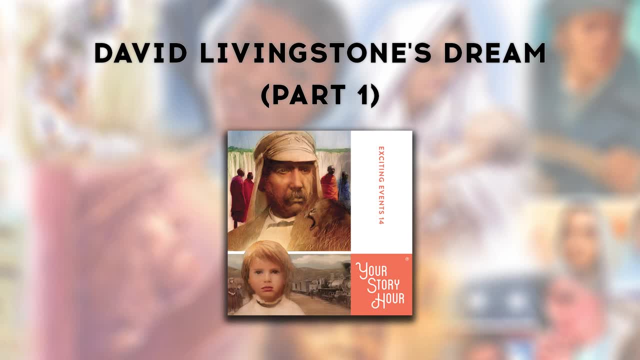 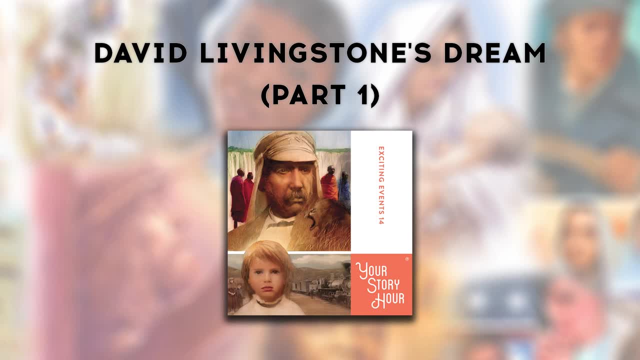 David Livingston's Dream. David Livingston's Dream. David Livingston's Dream. David Livingston was born in Blantyre, Scotland, March 19, 1813, the second son of a poor family whose father, a devout Christian, sold small packets of tea door-to-door as a way to support his family. 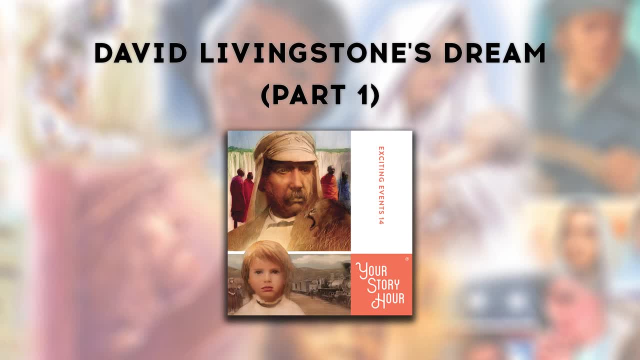 Eventually there would be five young mouths to feed as more brothers and sisters were added to the family circle. Unfortunately, given the pittance father earned, it soon became necessary for John, the oldest boy, and David, at age 10, to go to work in the cotton mill where they could earn a few pennies each week as piecers. 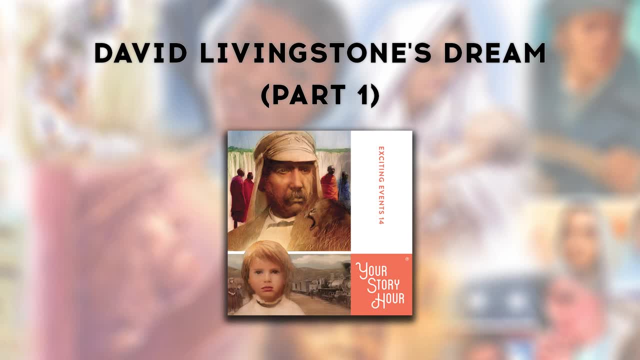 It was a job performed by scores of children who crawled around under the spinning machinery for 14 hours a day to quickly tie together any broken threads before they could be woven into cloth. The Livingston home was a single room on the third floor in a tenement called Shuttle Row, which sat on the banks of the Clyde River very near the cotton mill. 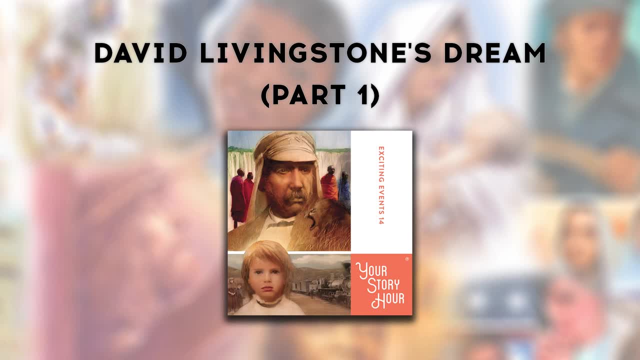 The boys' day started at five in the morning. Come my laddies, time to get up. Your porridge is almost ready and then it'll be off with ya. All right, Ma, Oh, Davey, another day crawling under the looms, hour after hour after hour. 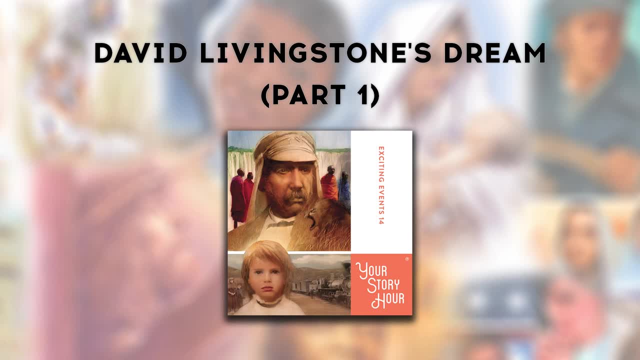 And trying to be fast enough not to get whipped by one of the weavers. Those leather straps they swing can really sting And leave welts. At least we can help with food, John. without the money we earn, I know, I know We'd all be starving. 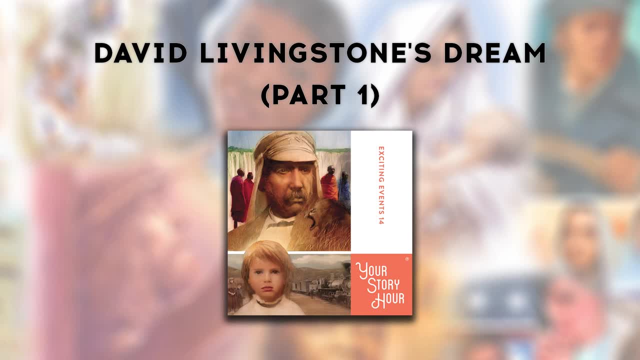 Hurry up now, you two. Your dad has already left for Hamilton to sell tea there today, But not just to sell tea. His pockets are stuffed, as usual, with gospel tracts. As you know, he views sharing Jesus with his customers as his true business in life. 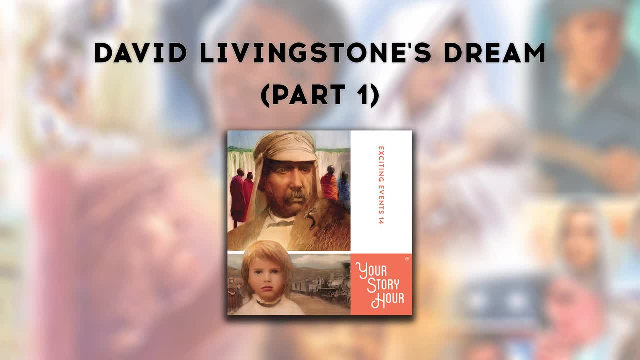 But up now, laddies, Look lively. All right, Ma, We're up Now today. Davey Aye Ma, This morning you can read our Bible verse for the day. Why doesn't he just quote one from Psalms 119?? 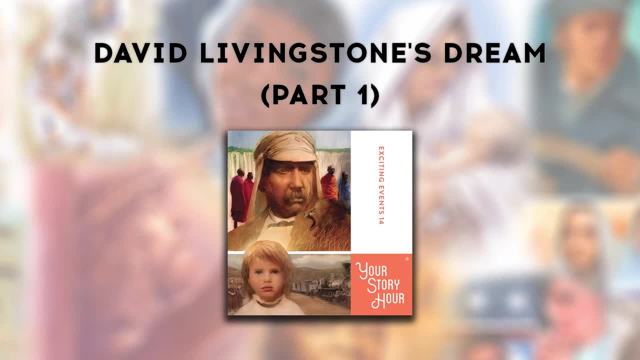 He knows it all by heart, all 176 verses. Indeed, he does. I wanted to win the prize and I did A Bible. And only nine years old when you did it, you was Ah Davy. your da and I are so proud of you memorizing God's word. 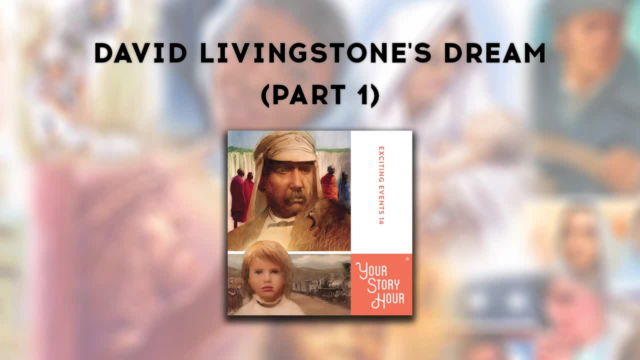 Oh, hurry up now, you two, You canna be late to the mill. As the months and years tumbled by, David continued the exhausting work as a piecer amidst the clanking looms and spinning spools at the mill, from six every morning until eight at night, 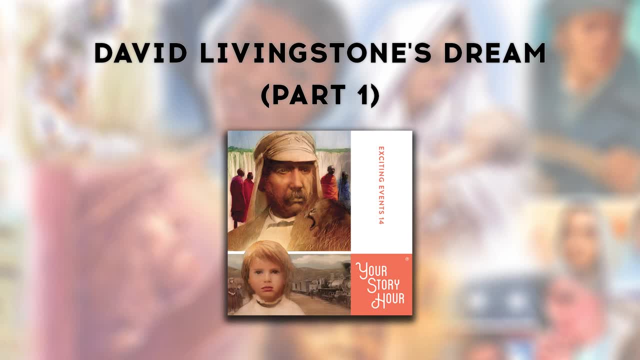 except on Sundays, when the mill was closed and the entire family walked three miles to Hamilton for church Afterwards. David loved to roam the fields and, using books borrowed from his grandfather, he delighted in identifying plants and flowers. Look what I found, John: a little clump of Campanula. Scottish bluebells. 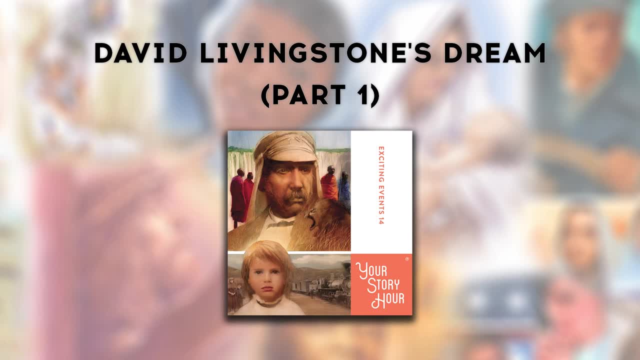 And then, come Monday, it was back to the mill again. However, every night after work, David was one of the few who took advantage of a special school set up for working children, which met from eight to ten at night, And even after he arrived home, he would open his books and study until his mother would tiptoe her way around all the sleeping figures on the floor to David's side. 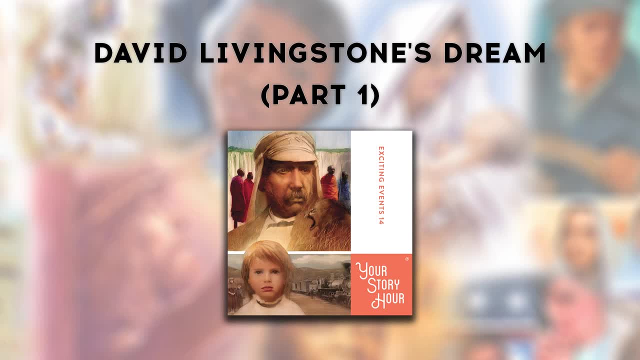 Oy, laddie, you do your Scottish Highlander heritage proud, learning as you do. But the fire's grown dim and it's already midnight, so give me your book and be off to sleep with you now. Even at the factory, faced with the endless routine and noise, David kept his mind active. 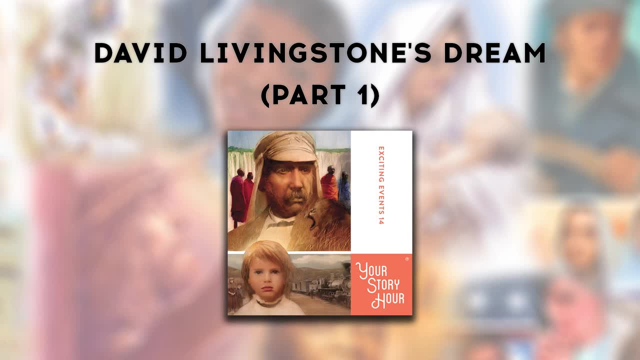 He had learned to read at the age of six and now he used every spare minute to improve himself, in spite of constant teasing. Look there, Maggie, it's that David Livingstone reading again. See, He has another book propped up beside the spinning jenny. 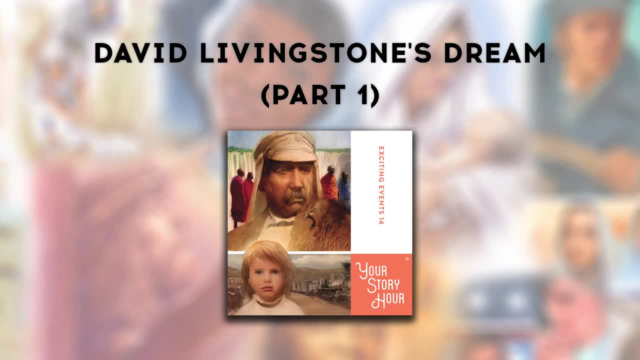 Just watch, I'll take aim with this big bobbin and throw it away. and there, Good shot, You hit the book square and knocked it to the floor. He's a strange one that David always. Hey, you two get to work. It's just what's so funny to you now. 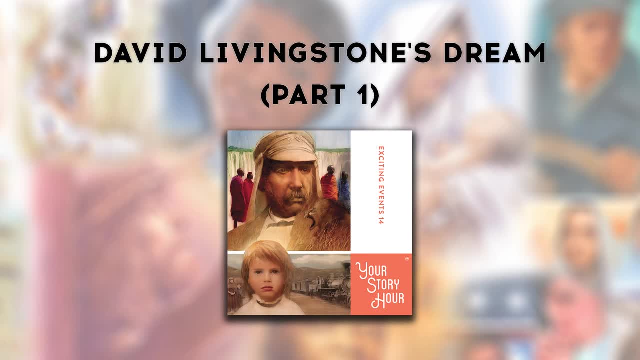 It's him, sir Livingstone. He likes to read books. What's this Livingstone Reading while you're supposed to be working? But, sir, I never miss a broken thread. And just what book have you here? Latin? This is a Latin grammar book. 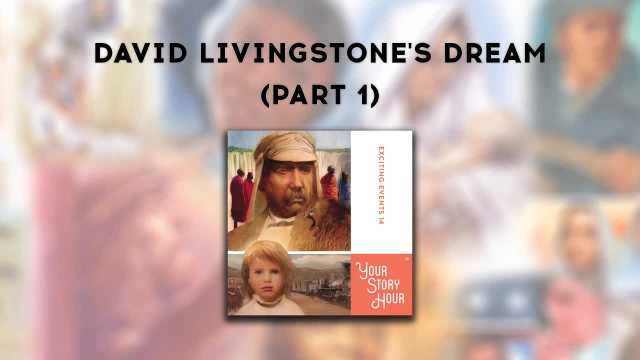 Aye tis, sir, I'm learning. And how long have you been Studying, Aye Latin? Not always Latin, sir. Other books too, But I want to learn about. well, everything A little good it'll do you, Livingstone. 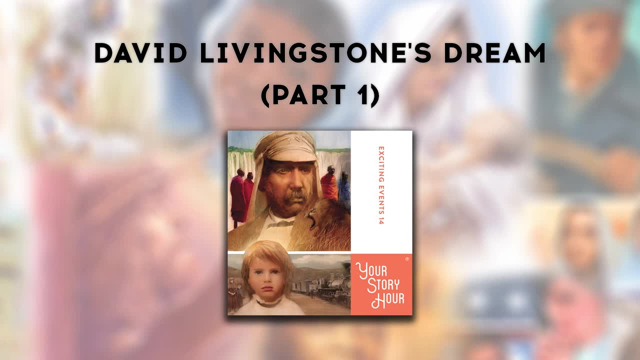 You was burned to the mill, and at the mill you'll stay. Just make sure you never miss a broken thread And don't let me see Another book. Now it's back to work with you. David solved his book problem by finding a little space behind the machinery where he could prop a book for quick glimpses while working. 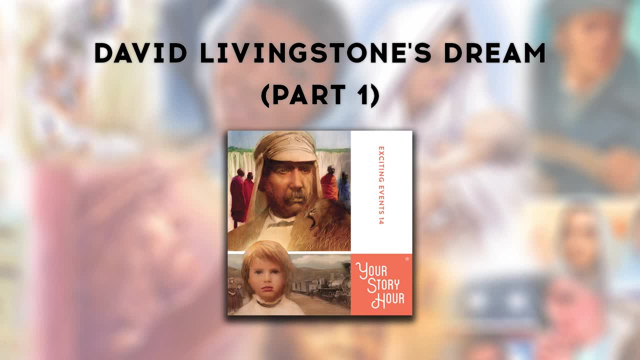 In fact, through the years he read and studied many books, including one written by Charles Gutzlaff And Ma the author told all about his two voyages along the coast to China. How he went. Mr Gutzlaff was a medical missionary, you see. 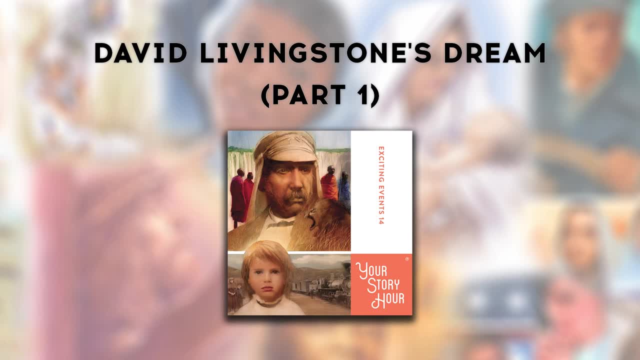 To China Aye. He shared Jesus with the people as he treated their diseases. That's what I want to do with my life, Ma. I want to tell people about Jesus, the one who died for us all while I helped them as a doctor. 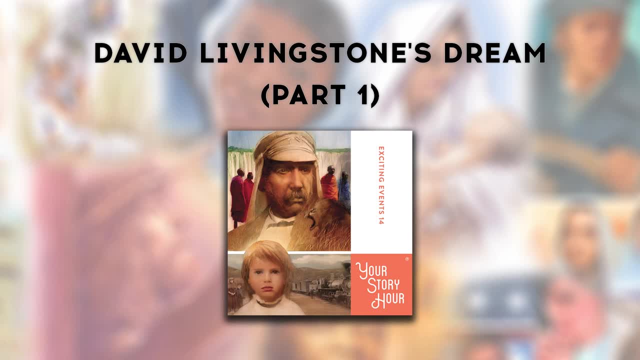 But Davy how. You have no money, We have no money. How can you ever Go to university, Earn a medical degree? Aye, I don't know, Ma, But my dream is to go to China as a medical missionary. 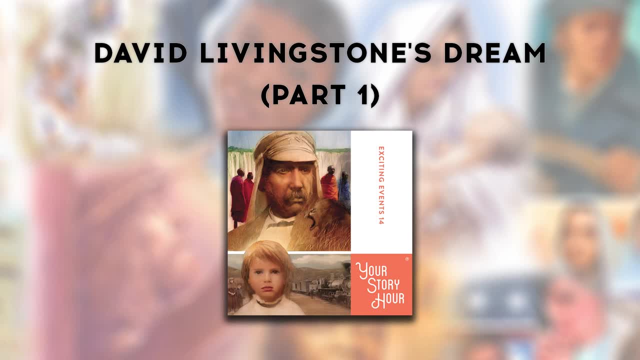 And somehow, By the grace of God, I will. Shortly thereafter, David was promoted to the position of spinner at the mill, which came with a slight raise in wages, And for the next four years, until he was 23 years old, he scraped and saved every penny. 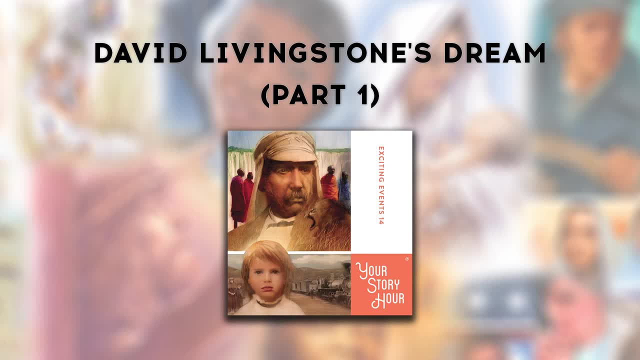 Then, in 1836, he was off to the university in Glasgow. Two years later he was accepted on probation by the London Missionary Society and sent to their missionary training center near London Where he was assigned to live with other students in the home of Mr Cecil, a minister and instructor. 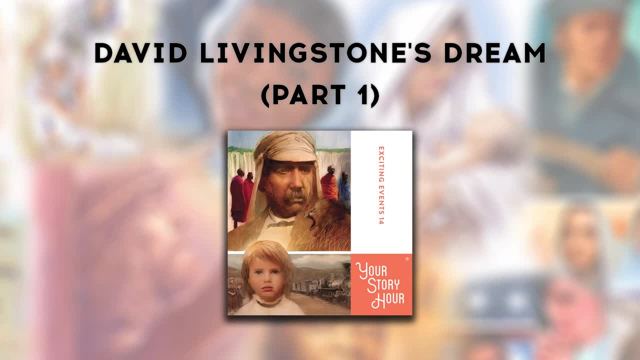 While here, as students, you will learn many things, practical as well as educational. You'll need to develop skills to survive in the uncivilized corners of the globe. At the same time, as part of your training, you'll be writing your first sermon. 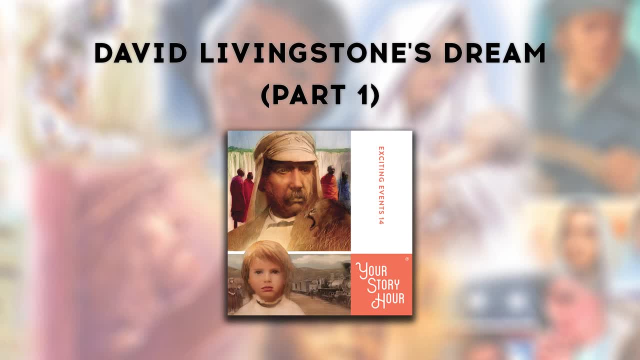 which you will be expected to successfully deliver by memory To congregations in nearby villages. Your speaking abilities will be evaluated by the board of directors before you can graduate from your apprenticeship here, David had no problem with the practical skills, but speaking in front of others proved to be more difficult. 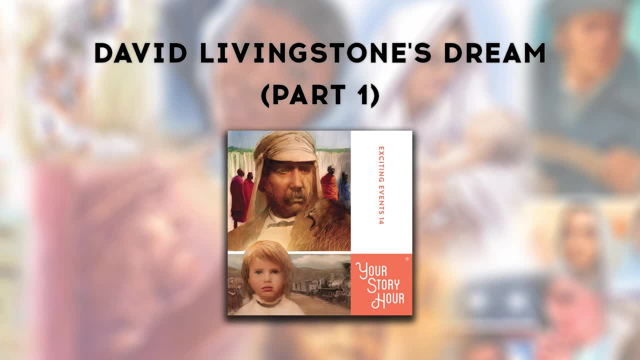 When it came time for him to deliver his first sermon, he, who had memorized the 119th Psalm as a nine-year-old, stood in front of his audience and froze: Friends, I, Friends, I, I. I have forgotten all I had to say. 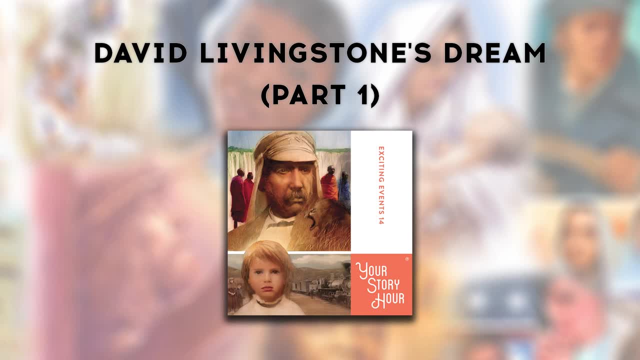 Turning quickly from the pulpit, David ran from the church and tramped through the night in utter despair. Oh God, how could I forget? How could I fail? The board will never approve me now- Never. However, although David did fail his first term of apprenticeship. 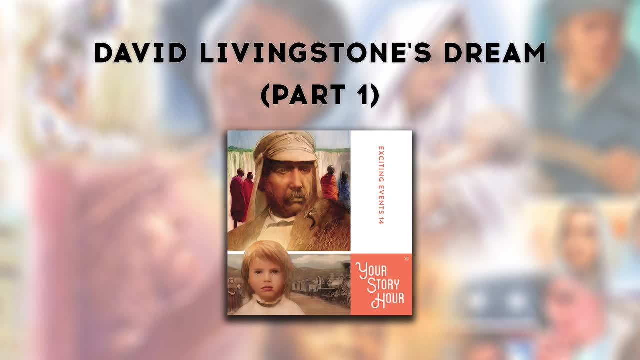 the mission board finally decided to give him another chance, And when he stood before them the second time- Livingston. you have now successfully completed your apprenticeship, which means that we will send you back to London to complete your medical training at our expense. 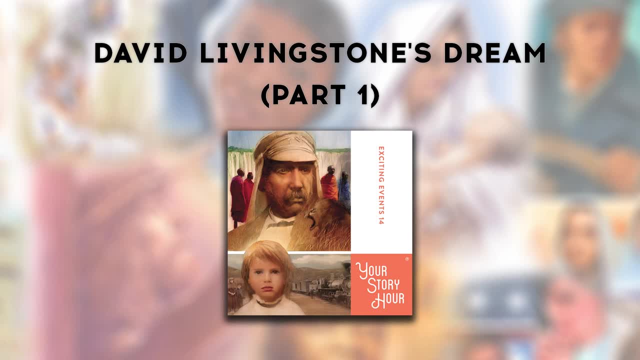 Here now was an area where David excelled with ease. He was popular with his patients and his excellence in the field of medicine was recognized by established physicians who generously offered him a position to practice in London. But David's goal was set. 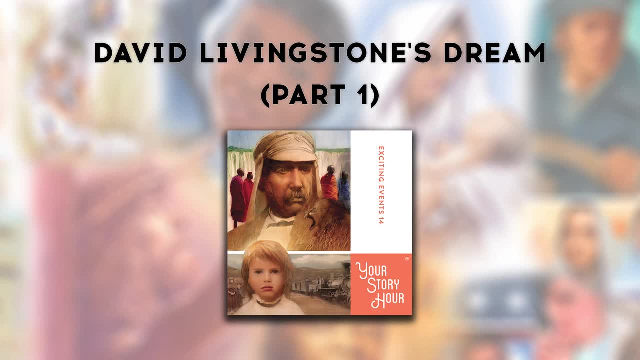 He would dedicate his life to reaching those in the most dire need of his help. He would go to China. However, I'm sorry, Dr Livingston, but because of the opium wars that have recently broken out in China, many of the London Mission Society are no longer sending medical missionaries to that country. 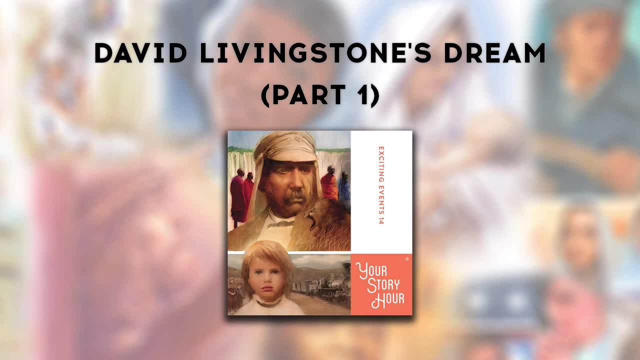 The news was a definite blow to David's long-held dream. And then one night, he happened to attend a talk by Robert Moffat, a missionary with tales to tell of his experiences in Africa. Yes, friends, I've had a bounty of 100 pounds sterling put on my head. 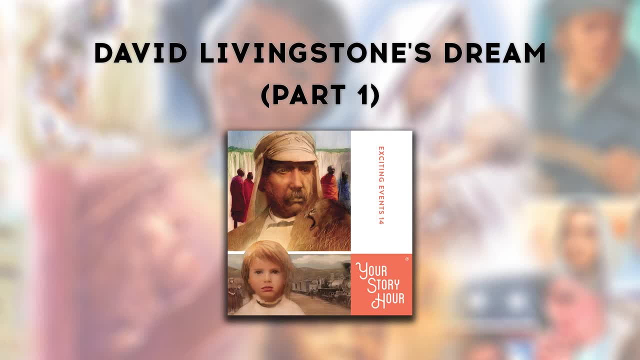 I've traveled many miles by ox cart from our home base in China to visit Kuruman, but there is still so much yet to be done. The great heart, the massive interior of Africa is still silent. I have seen, in the morning sun, the smoke of a thousand villages. 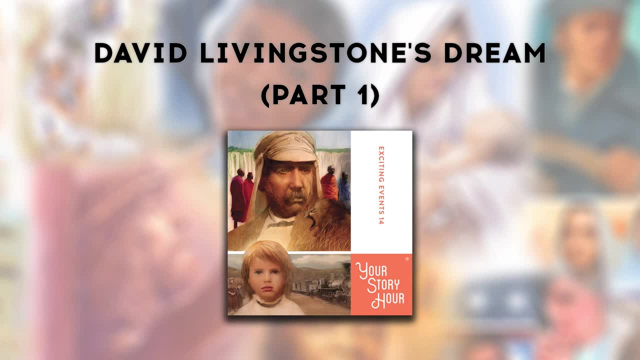 where no missionary has ever been. In that instant, David Livingston's dream changed direction. His heart was moved by his desire to take the gospel to Africa's interior. He was shocked as he learned more about the terrible slave trade in Africa, And his spirit of adventure was ignited when he looked at the map. 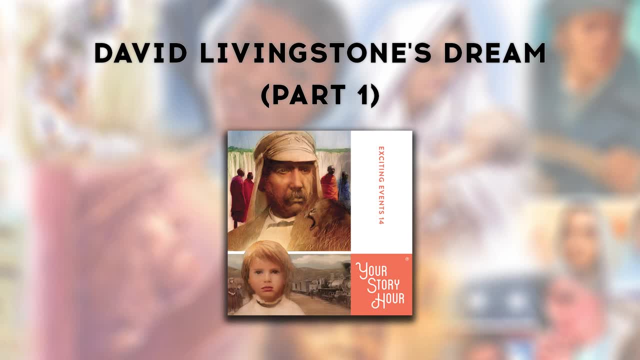 displaying the vast blank section in the center of the African continent. Hmm, It's marked as unknown, Unknown, Unexplored, Unmarked. Yes, Africa is the place for me. Ah, it's such a good feeling to know your special place, isn't it, Aunt Nikki? 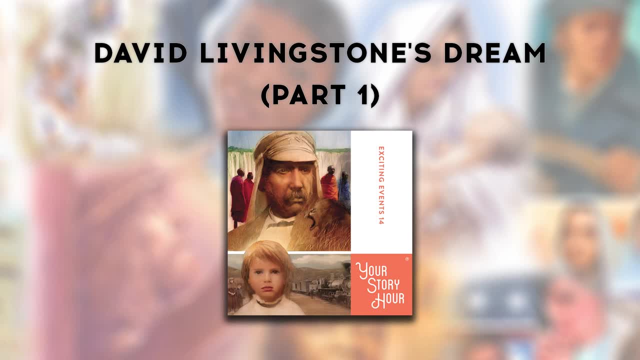 Oh yes, Uncle John. Boys and girls, did you know that there's a special place just for you on the Your Story Hour website? It's called Kids' Corner, and there you can find Clubhouse magazine full of interesting stories and jokes and games. 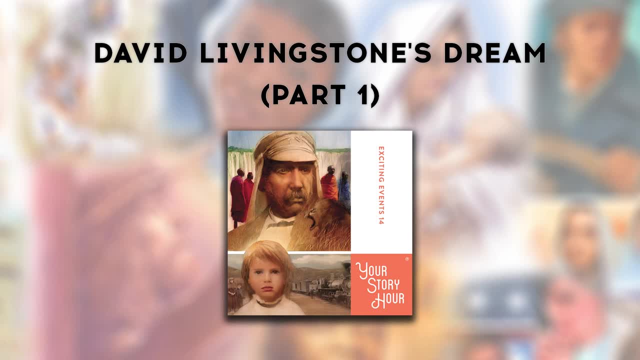 There's adventures in the Holy Bible, a fun dive into God's Word. There's a coloring book that goes along with a classic story, The Raven and the Ring, And you can even stream the story for free while you color. Check it out at YourStoryHourorg. 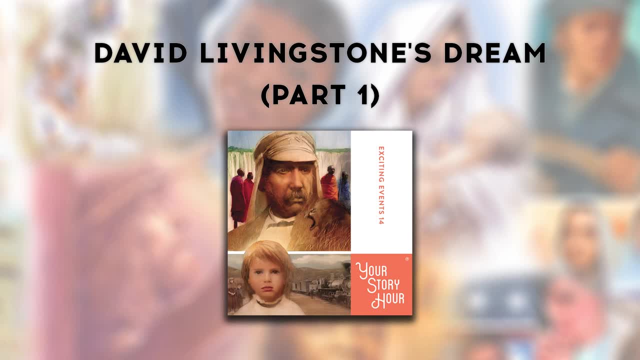 Listen now as we continue with the story called David Livingston's Dream. On December 8, 1840, the HMS George slipped out of port in England and began its voyage towards Africa. Aboard was 27-year-old Dr David Livingston. 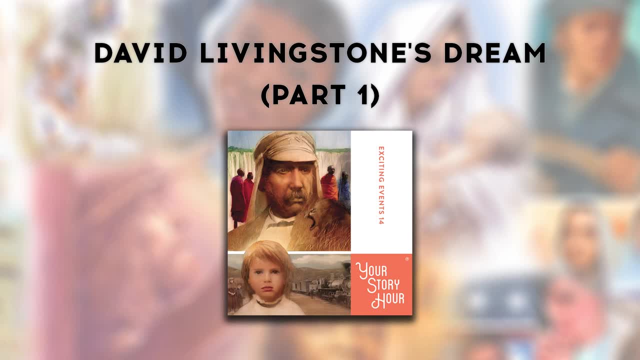 eager to embrace his African adventure as a medical missionary. Unfortunately, the ship encountered some difficult times thanks to a violent storm at sea. However, during the calmer moments, the ship's captain willingly taught David how to navigate, a skill which would later help him map much of Africa's interior. 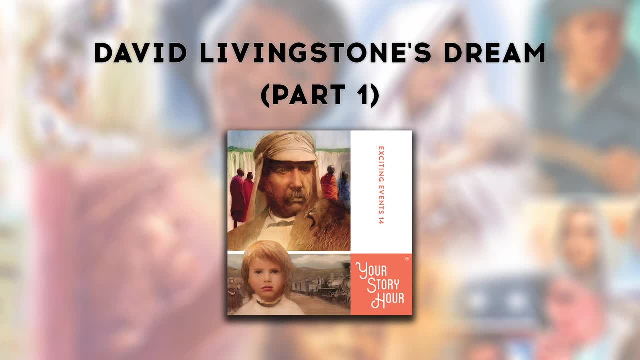 And now, Dr Livingston, since you've mastered the use of the navigational tools: the sextant chronometer, The book of mathematical tables- Yes, that too. Anyway, let's meet here at the chart room tonight and I'll show you how to navigate by the stars. 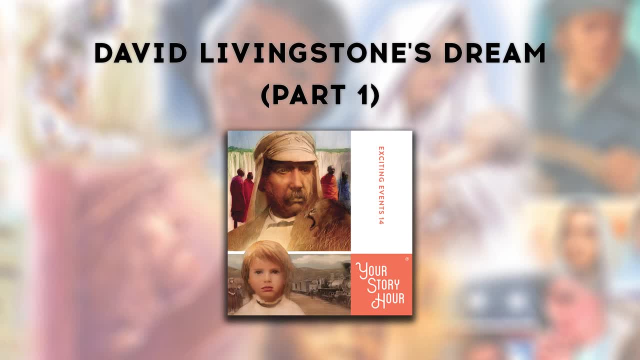 After several months, the ship pulled into Port Elizabeth, near the southern tip of Africa, And from there, accompanied by fellow missionaries, William Ross and his wife, along with several African guides, David, traveled 600 miles by ox cart to Curramon, Robert Moffat's mission compound. 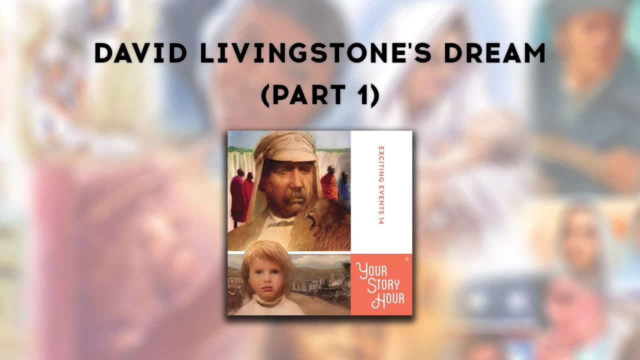 After ten weeks of travel, they arrived on July 31, 1841, and were greeted by Roger Edwards who, with another missionary, had been left in charge until the Moffat family returned from their furlough in England. Knock knock. 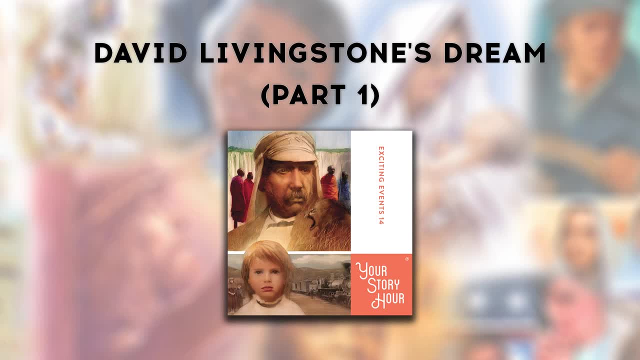 Come. So, Dr Livingston, all settled, Bags unpacked. Yes, thank you, Mr Edwards. None of that. now Just call me Roger And you can call me David, All right. Well, as you can see, the Moffats have developed. 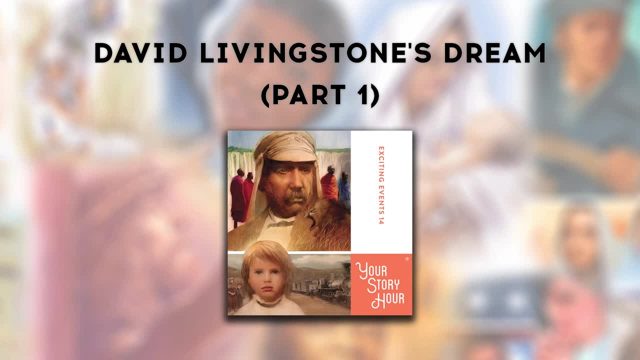 quite an extensive compound here after 20 years. Yes, comfortable housing, shady verandas, fruit trees, a village for the workers, even a blacksmith shop, And don't forget the new church. I'm surprised really. I actually wondered how Mrs Moffat has survived here. 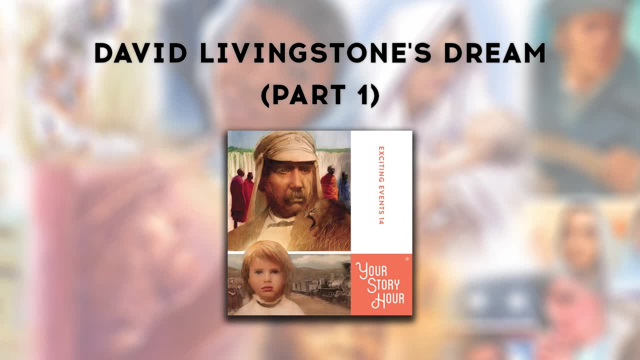 Africa is after all called the white man's grave, And for a woman, Ah yes. the compound is like a little piece of England, And the Moffats have raised their family here. Mary, their oldest and the other children were all born in Africa. 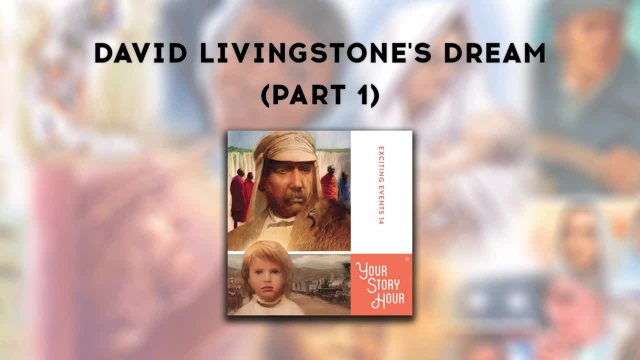 Has Pastor Moffat ever gone inland at all to try to reach the natives there? Yes, a bit, And he's learned some of their languages. But mostly the work has been centered around here at Curramon, I see. So I 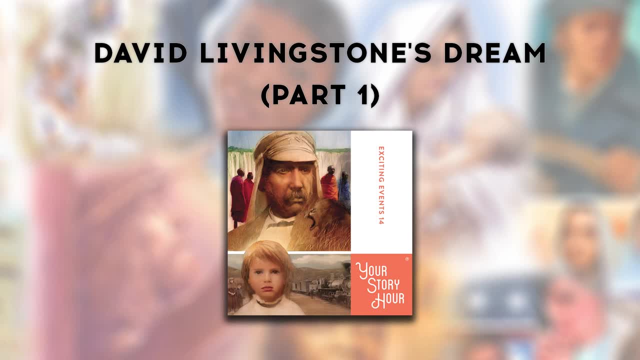 I see a group of the people gathered outside there, just beyond the veranda. What's that about? Well, Doctor, the natives are very excited to learn that you are here, A real medical doctor, The first ever to come to the mission. 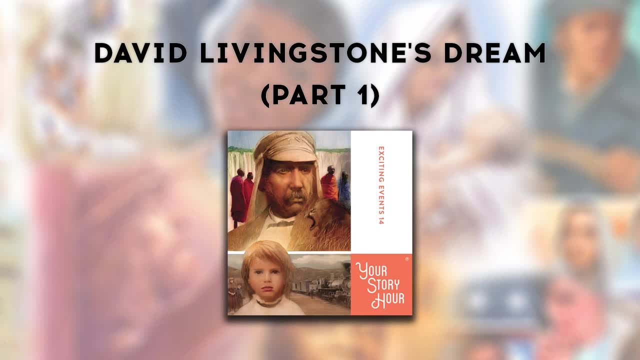 They're bringing their sick for you to see, But I'm not set up yet. My supplies are still in boxes. Before long, however, David was busily tending the sick who, it seemed, arrived in a never-ending line, some coming from more than a hundred miles away. 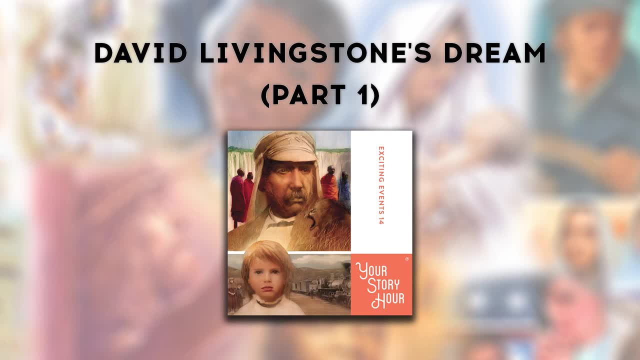 Hmm, It looks as if this wound goes all the way to the bone: High fever, jaundiced eyes, swollen abdomen- Clearly an infected snake bite. I just hope I can save his leg Soon, overwhelmed by the sheer numbers of people. 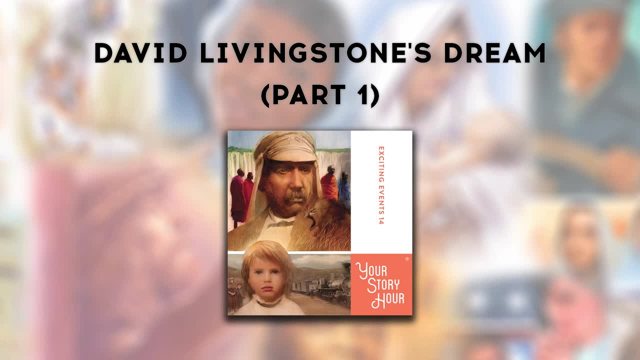 needing medical attention. David trained a few of the African Christians at the mission to care for the more minor cases, But within weeks, even with their help, he knew he must make a decision. It seems that if I'm ever going to accomplish my true mission. 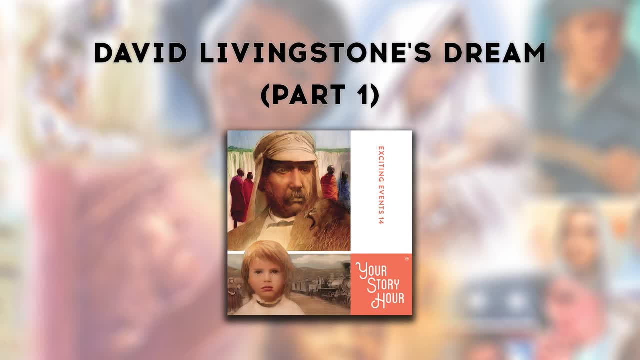 I'll have to break from being just a doctor, a veranda missionary, so to speak, and push forward with the Gospel far into the unknown interior. And so, accompanied by his family, an African guide named Pumari and several others, 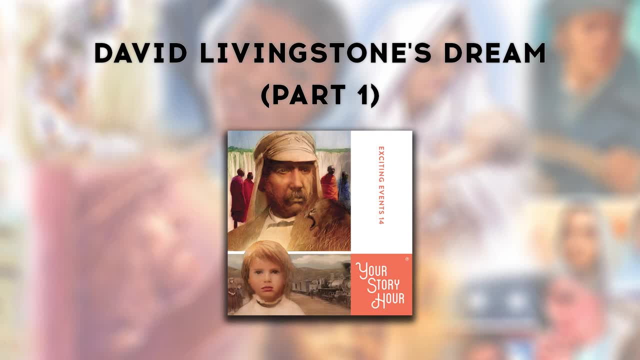 David, along with Robert Edwards, was soon on his way by ox-cart caravan northward from Kuruman. He quickly found that there was much to learn about African customs. What's this, Pumari? The village is completely empty. Where is everyone? 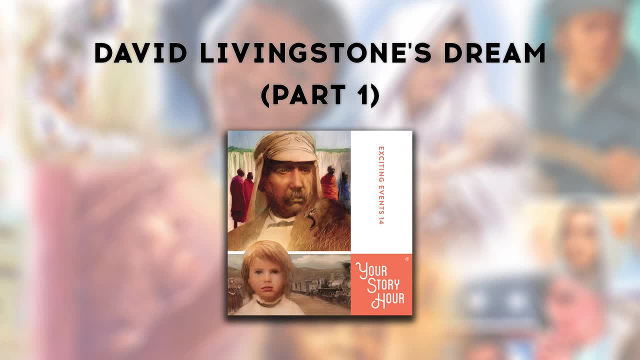 They have seen you coming and are hiding. They are afraid of white men. So what can we do? I will go and find them. I will go ahead to the villages before we arrive. Will that work If I take beads and cloth as presents? 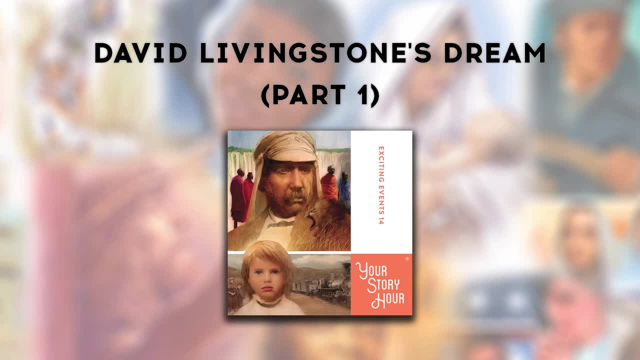 and tell them you come in peace. that is the polite way. Well then, that's what we'll do. Over the next few months, David visited a number of villages, and often the villagers were afraid and suspicious of him at first. 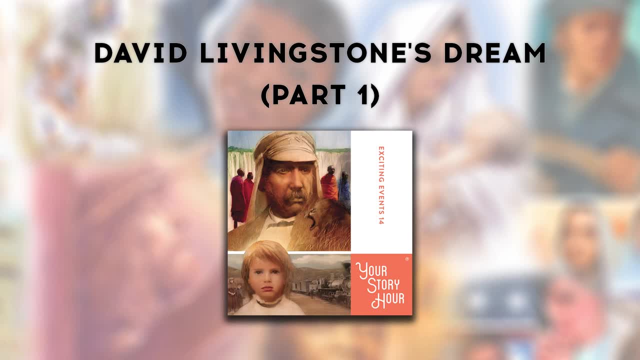 some of them even confronting him with weapons. He could see how important it was to learn their languages as quickly as possible. He also learned how difficult travel could be, with the enormous distances to be covered, along with the dangers involved. He could often hear wild animals stalking nearby. 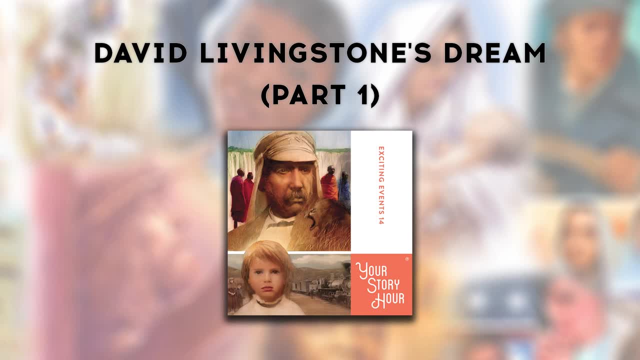 but even some of the minor annoyances were challenging as well, One morning as they were awakening in a hut which had proudly been offered to them by the village chief as overnight accommodations. Oh well, Roger, not a bad night's sleep all in all. 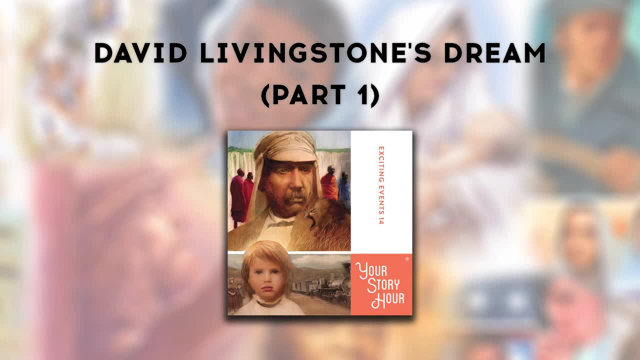 But what's this? Look here, These little blue orbs. So many of them between my fingers. Oh no, I have them too. Tampon, I should have thought We slept directly on the dirt floor. Tampon- African ticks. 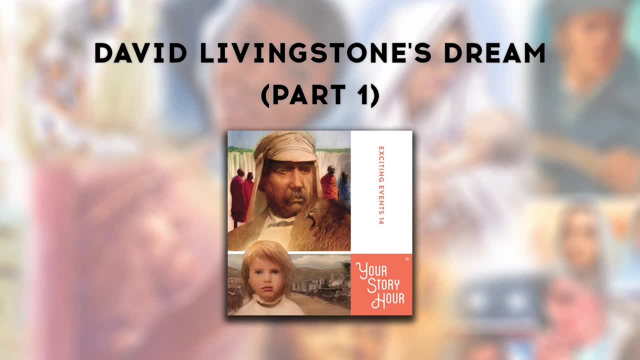 They live in the soil. No, no, don't try to pick them off. They're firmly attached, sucking your blood, and if you pull them off, Ah yes, ticks. you said. If I pull them off, their heads will stay buried in my skin. 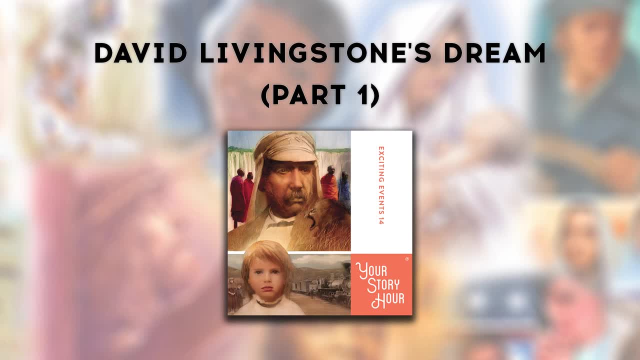 and infection will set in. Exactly. We'll have to touch each one with a hot needle. Hopefully they'll let go and fall off There. Finally, they're all gone. You know, David, while we're in this area, 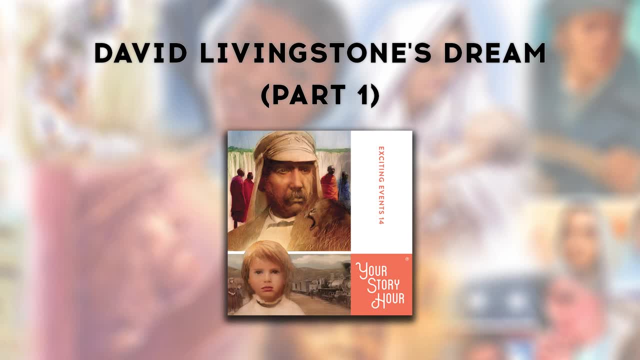 we'll have to find a way to sleep off the bare ground. Hmm, I have an idea. Oh no, it'll have to wait. my friend Prepare to become violently ill. Within seconds, both men were outside on their hands and knees. 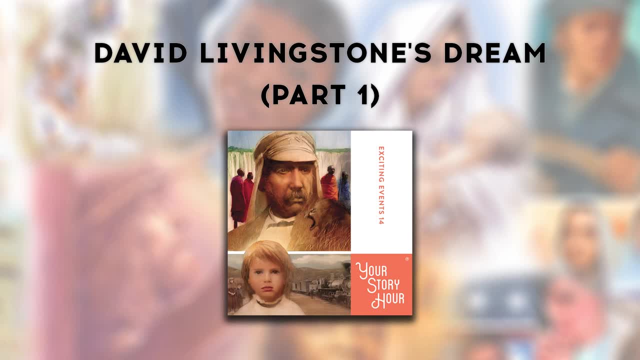 their stomachs, feeling as if they would turn completely inside out. It was several hours before they recovered enough from the poisonous tick bites to stand up. Then, still a bit wobbly, David spoke with the village chief Chief, as I have promised. 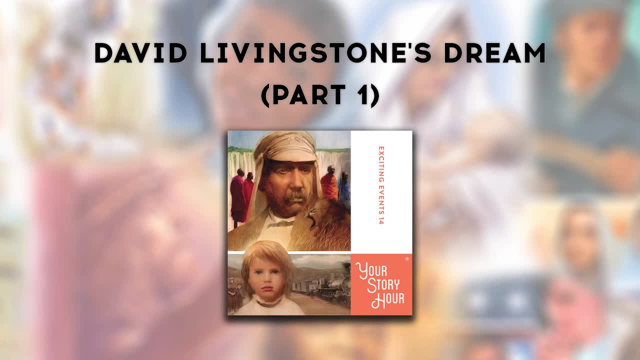 I will treat all the sick in your village, but I need your help. Speak, Speak. I know your village. shaman has his own hut. Ah yes, A shaman's hut holds many, many secrets, Exactly, And for my medicine to work best, 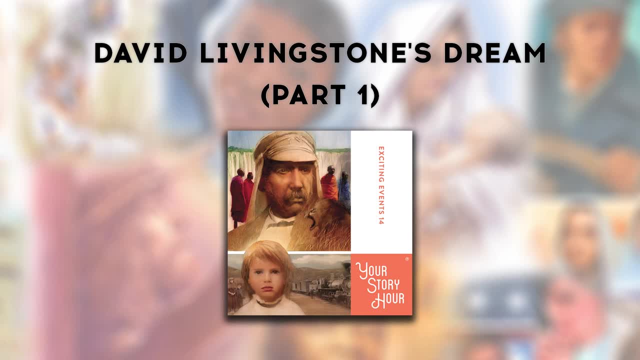 I'll need my own special hut as well, my tent to serve as my clinic. I understand You are a white shaman with your own secrets. Come, I will show you where to put your tent of magic. All right, Roger, this is the spot. 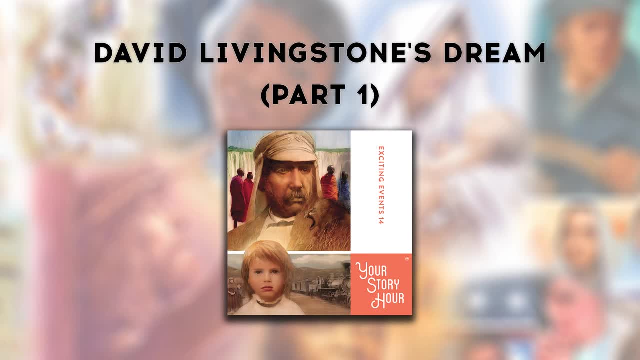 First we'll scorch the earth to kill the ticks, then lay our tarp over it and put up our tent. We can use it as our own living quarters and sleep here as well. Fortunately, the tent arrangement worked well, and once David had treated the villagers, 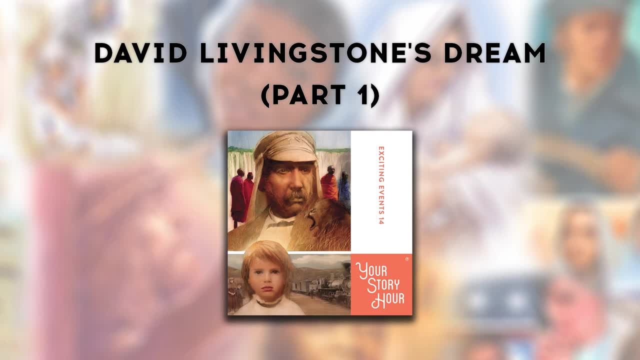 and shared the love of Jesus with them. it was time to move on and visit more tribes, After leaving one village where David made friends with Chief Seschel by treating him with his medicine, Chief Seschel by treating his sore eyes. 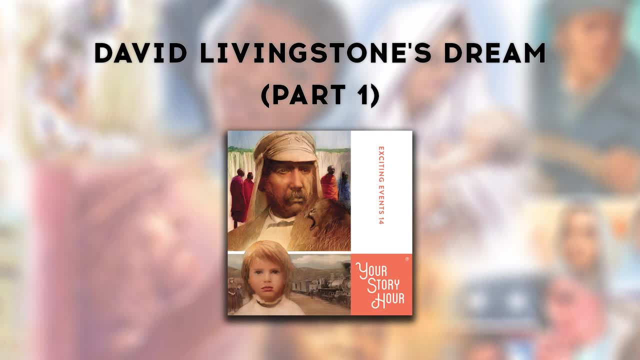 the caravan traveled about ten miles southward back toward Curamon before making camp for the night. Suddenly, David heard a curious sound. Roger, listen, What is that? It sounds like someone crying- Yes, like a child. And it's coming from there, under our wagon. 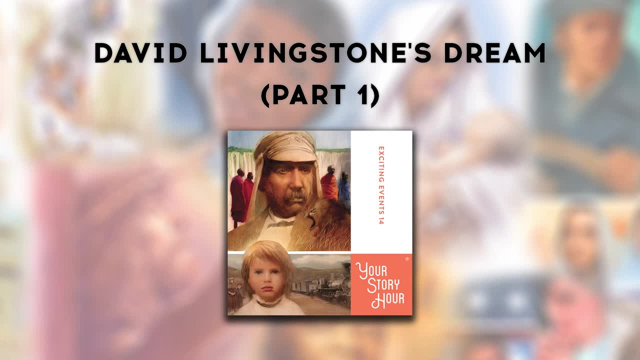 We'd better take a look. Why look crouched underneath? It's a girl. Hello, Yes, you Come. come, it's all right. She looks terrified, That's right come. Ah, good, Here, let me help you stand up. 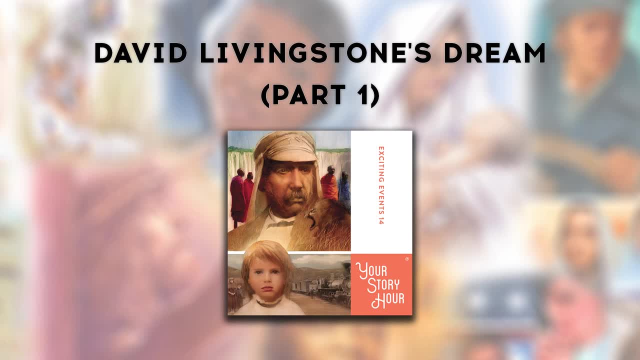 Why she must have followed us all the way from the village and then hidden under our wagon. Don't let them take me. Who, Who are you afraid of? They want to sell me, Sell you? Uh-huh, David. she can't be more than ten or eleven years old. 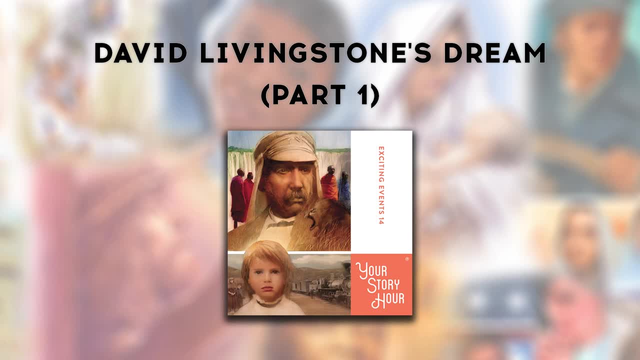 Please don't send me back. My mother died, My father died, And then my sister. I've nobody but my uncle, And he's- Yes, He's- going to sell me as a slave. Oh, dear child. Now then, first things first. 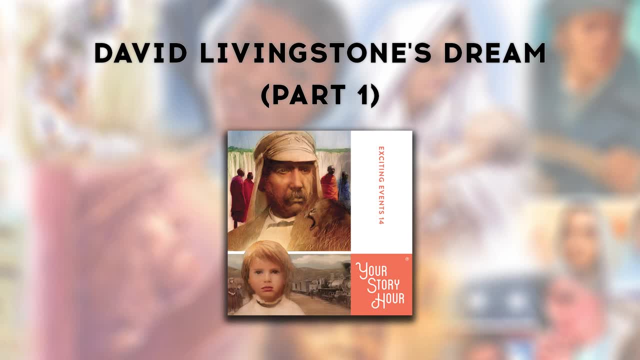 You look very hungry. I'll ask Pomare to get her something to eat. Pomare, Look, he's already headed this way And with someone who doesn't look too friendly. Oh no, it's a warrior from my village. 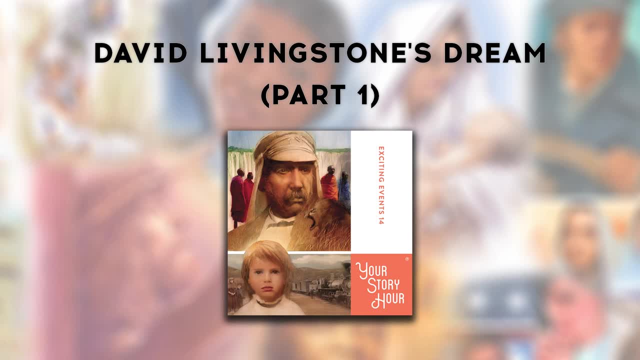 No, I tell you she will not go with you. She escaped And she wears many beads. Her uncle probably loaded her with beads to make her more attractive, to bring a better price when he sells her. Ah, I see Pomare. 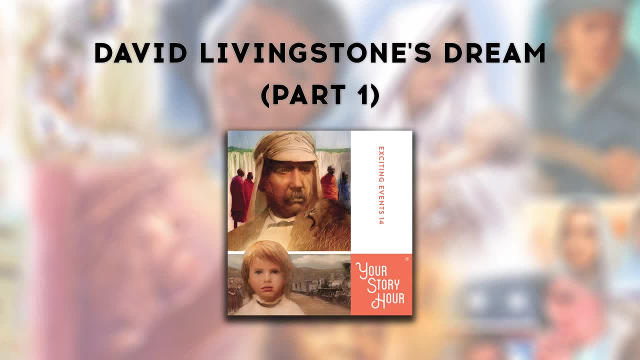 Give her to me Now. now there's no need for your gun. I take her. You come with me. Wait, You see, she's just a girl. No good to anybody, Skinny, No money, Nothing, Except for the beads around her neck. 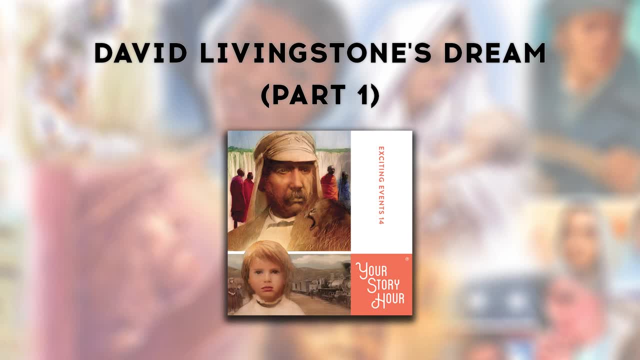 Yes, Many, many beads. So, yes, Here, let me help you take them off. All right, Here now You take these beads Instead of the girl. Good money And less trouble than the girl. yes, Take them all. 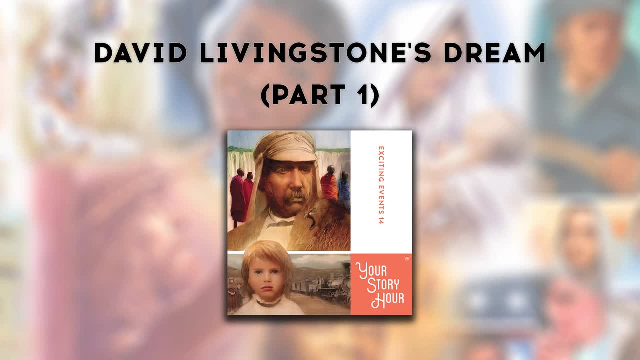 You keep her, I take the beads. Thus the crisis was avoided And the experience served as David's personal introduction to the slave trade so prevalent across Africa. I tell you, Roger, if they had sent 50 warriors, I would not have let them have her. 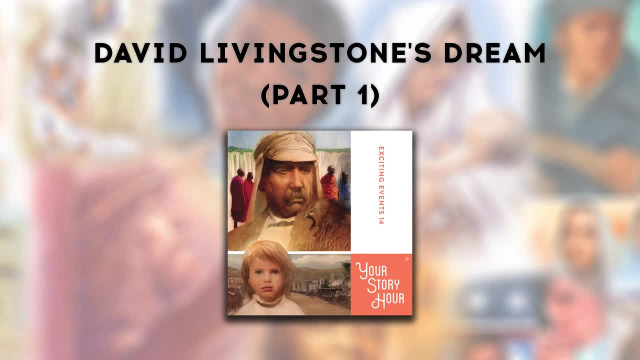 From that moment on, David determined to do everything in his power to end the practice of slavery. It would eventually become an overpowering passion in his life. For now, however, the caravan with the girl continued back to Curramon. 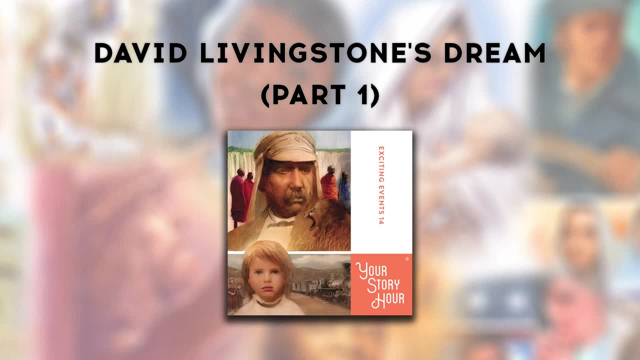 Then, discovering that Reverend Moffat had still not returned, David set off on his second excursion northward, this time with an all-African crew. They visited village after village, where David told them of Jesus, treated their medical needs and assisted them however he could. 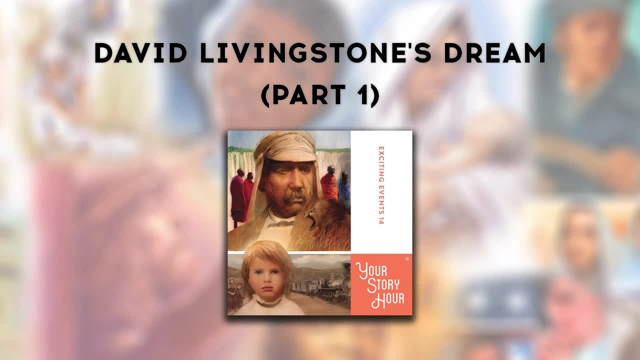 Chief Bobby, I think I can help. My witch doctor has already practiced his magic and still the rain does not come. The corn is dying Without it. we will die too. Well, I have a plan. What plan? Just bring everyone to the river. 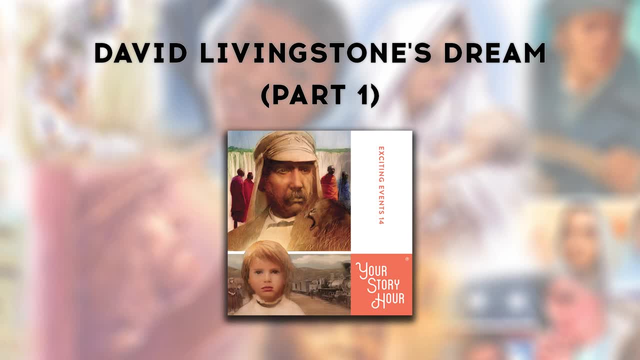 It's a bit distant, but together we'll build a dam. Then, since we have no real tools, we'll use sharpened sticks to dig a long way into the earth, all the way to your fields, As David and Chief Bobby worked together. 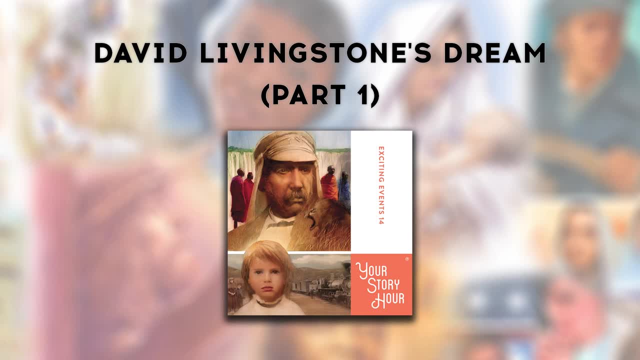 There, The last load of mud is in place. That should do it for the dam. Doctor. why do you come to help my people, Oh, Chief? let me tell you about someone else who came to help everyone. His name was Jesus, the son of the one true God. 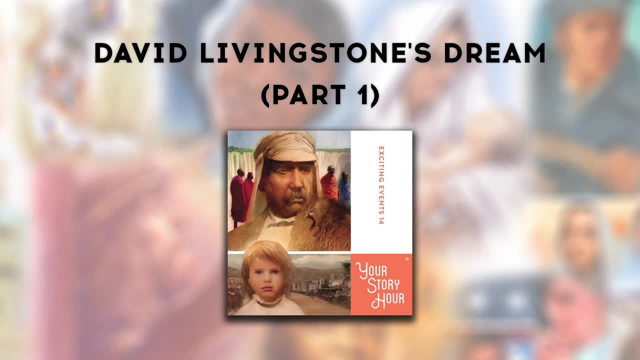 The God who loves you. Thankfully, David's irrigation plan worked. You have saved the corn. You have saved my people. Soon thereafter, however, David learned of a disaster: Chief Bobby had been accidentally killed by an explosion perpetrated by the village witch doctor. 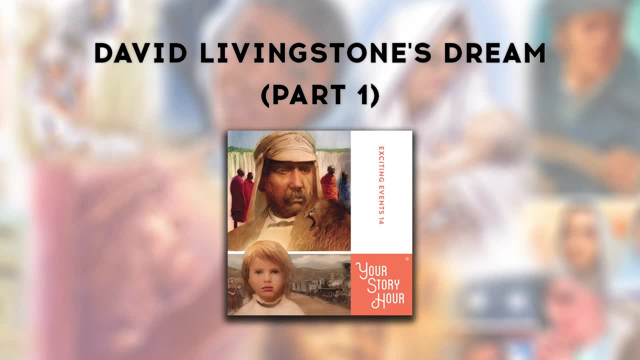 trying to get rid of evil spirits. I only pray that Chief Bobby accepted the saving love of Jesus into his heart before he died. As David continued to travel from place to place, trouble never seemed far away. In one village, for example- Lions, you say. 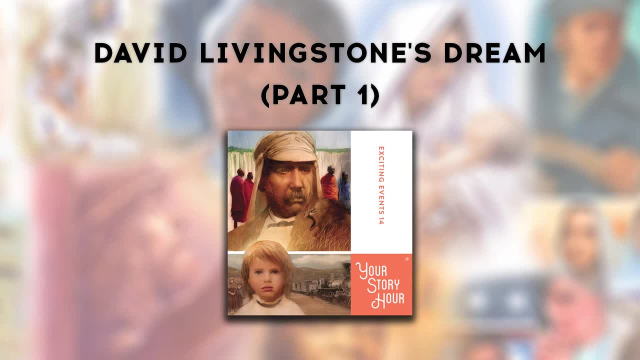 They're attacking the people of your village. Yes, attacking, But I've come upon many lions on that trail and when they've seen me, they've just turned and gone back into the bush. But these lions, they are now hungry for human blood. 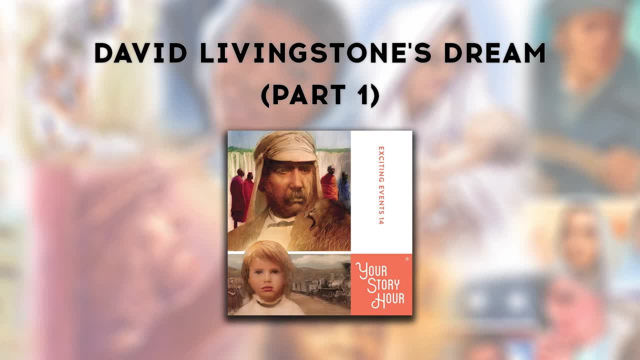 You must be careful as you travel. My, my friend, she, She, Yes, go on. She was working in her garden with her two children and the lions pounced on her, No, Yes, And before the men of our village could get there, 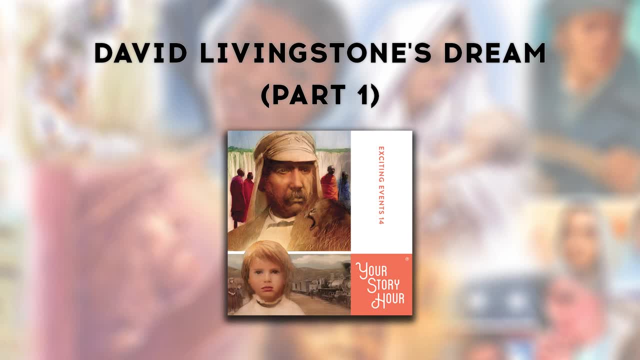 the lions, they, they, What. What happened They? they ate her. They ate her Right in front of her children. Oh no, The dreadful lion. The dreadful news tore at David's tender heart, especially as he heard the orphaned children. 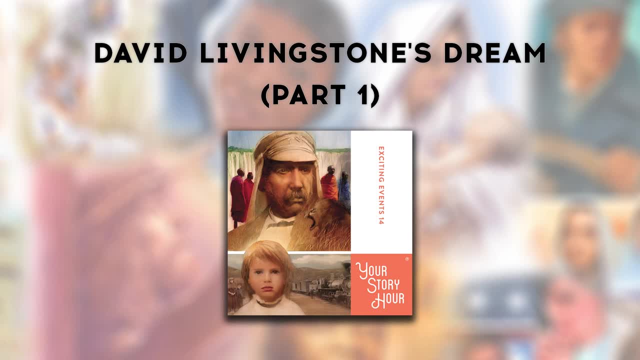 weeping into the night. He recorded the awful incident in his journal and later sent an anguished letter back home. Oh, if people in the civilized lands could hear the cries of the people, they would realize how much Africa needs help, And with every passing day.